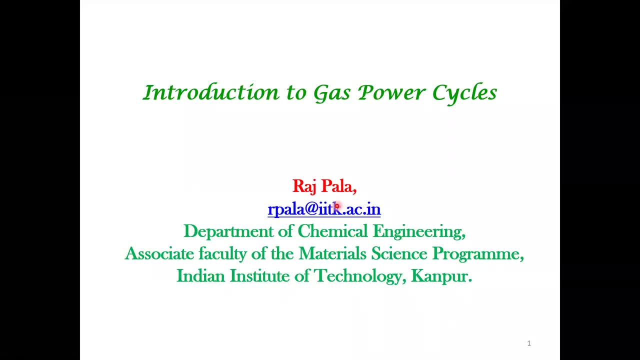 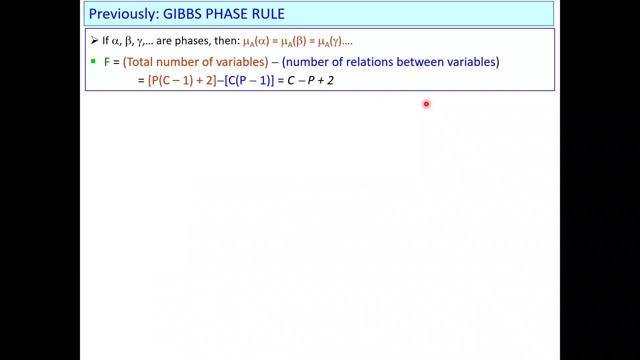 Welcome back. In this lecture we will look at gas power cycles. So we will take a few lectures to address issues of power cycle and this will be the first of these lectures. In the last lecture we had looked at Gibbs phase rule and it is instructive to look at the way we derive this simple expression. 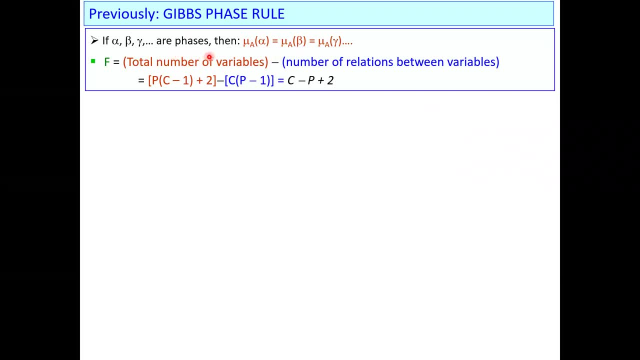 We considered multiple phases and there are different components in each of the phase and when they are in thermodynamic equilibrium, there is different components of thermodynamic equilibrium. There is thermodynamics, There is thermal equilibrium, mechanical equilibrium as well as chemical equilibrium. 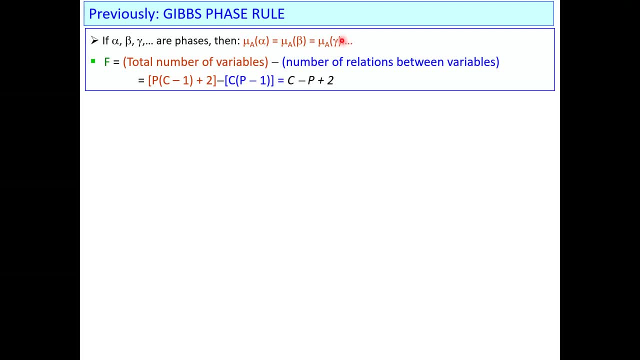 So this condition is the condition for chemical equilibrium. So the component A in phase one has this chemical potential. This is the typical symbol. mu is used for chemical potential, or you can also use g, small g doesn't matter. So this's the final condition for cal. 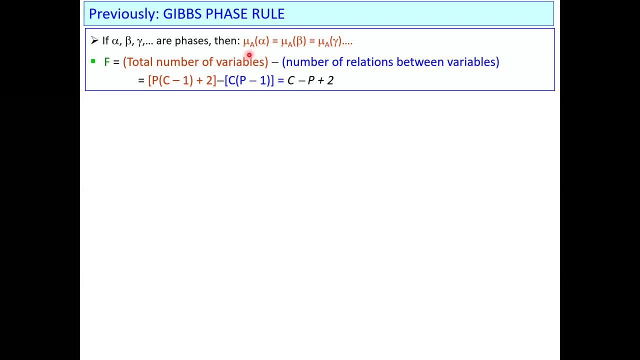 When is someChat A an equilibrium across all phases? When is there a certain chemical potential, the same chemical potential? when A is in equilibrium across all phases, then its chemical potential has to be the same across all phases, So similar constraint can be written for different components and so on. 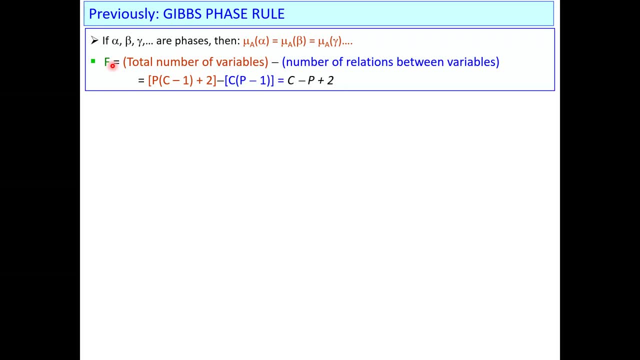 So F is the degrees of freedom. So the way we derive the gives phase rule is list out all the variables that is of relevance, So death, marry, the randomness or the ratio and so on of relevance, compositional variables as well as pressure and temperature, and then you subtract. 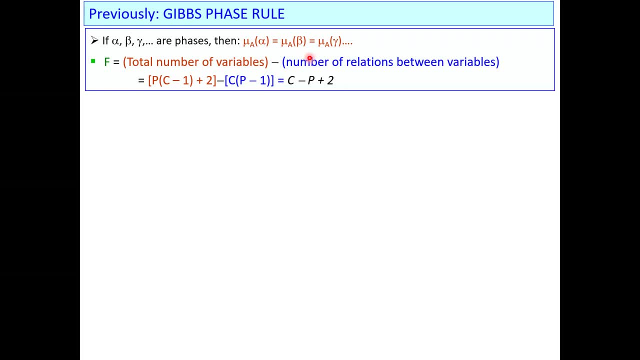 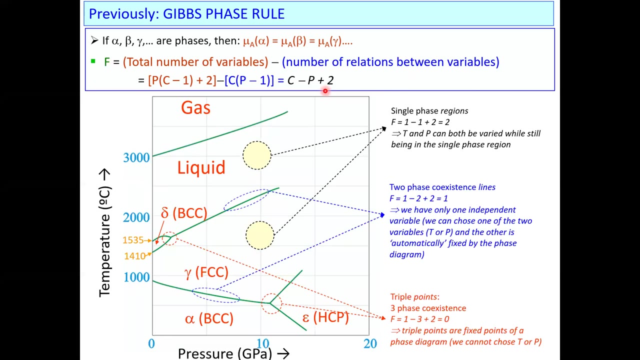 off the number of constraints with that you can derive the Gibbs phase rule. F is equal to C minus P plus two is a very, very useful, yet simple. so we illustrate a different aspect of it. I'm not going to go through the entire lecture, of course, so I'm just going to tell how we use Gibbs phase rule to. 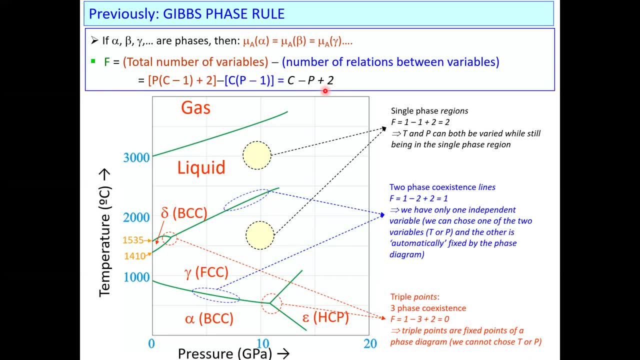 analyze a phase diagram. so phase diagram and material science often involves solids. here we think iron. as you can see, here the temperatures are rather higher and the pressure is also rather higher than what you typically see with liquids and so on. let's say water phase diagram and then we looked at different sectors of the phase diagram. so in this regime, what is the? 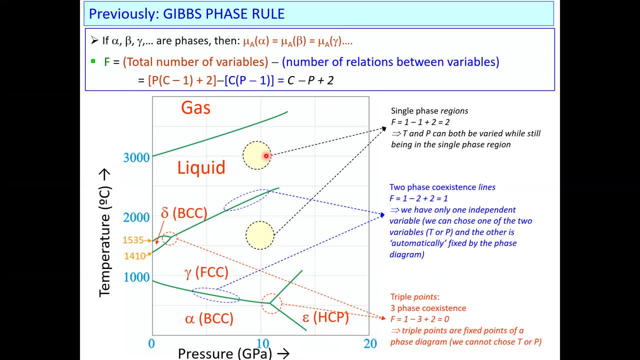 degree of freedom, the. here it's a unary phase diagram because the component is only one, the face is also one. so if we implement the Gibbs phase two- C minus P plus two- you get the degrees of freedom to be two. by that, what do you mean? that is like we can independently change temperature. we can, irrespective of the. 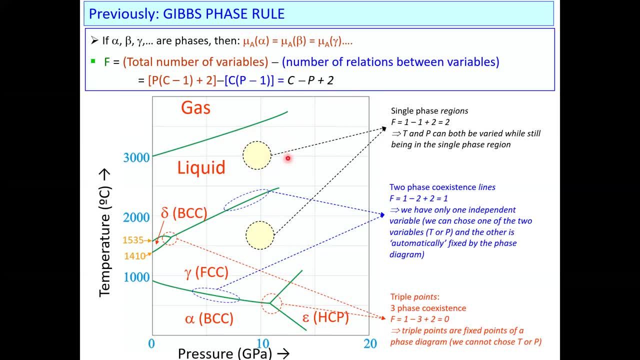 pressure and independently change pressure, and we remain in this regime. okay, so there's no phase, new phase that appears or disappears. so that is the same case here too. here component is still one unary phase diagram, but the phase is two. right, there are two phases that are in equilibrium: this phase and this phase. so if you implement the degrees of Gibbs phase rule, 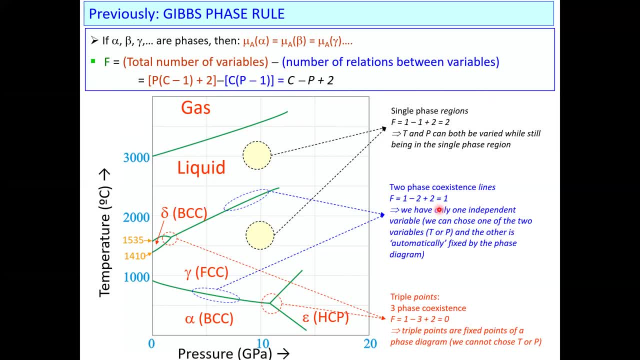 you get the degree of freedom to be one. so if I want to stay in this two-phase region, if I fix the temperature, or if I state the temperature, it automatically fixes the pressure. okay, so I cannot change it independently. I can only change one of them independently I can. 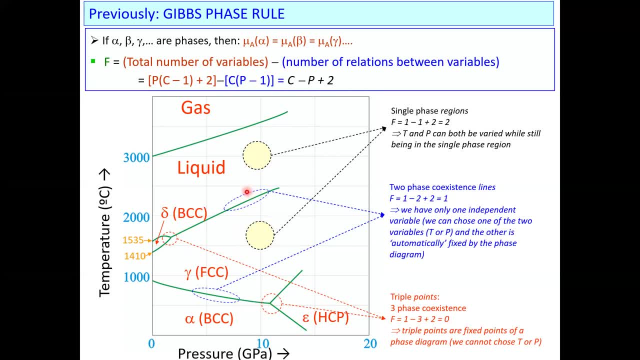 change the pressure, that means there's a corresponding change in temperature. okay, so that's what you mean by the degrees of freedom, to be one. and then there are other places where there are three components that are in equilibrium with each other. so there, the degrees of freedom is zero, right? so for this, 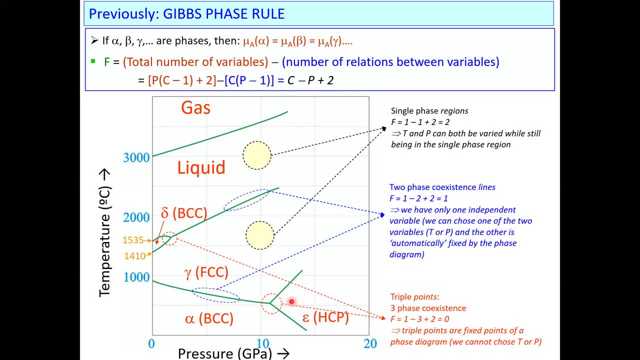 there's you. really, if you want these three phases to be in equilibrium, you really do not have any choice. the system chooses that temperature and pressure where that such three three phase equilibrium can exist. okay, so you should know how to use the Gibbs phase rule. it in different phase diagrams. let's move on to a new. 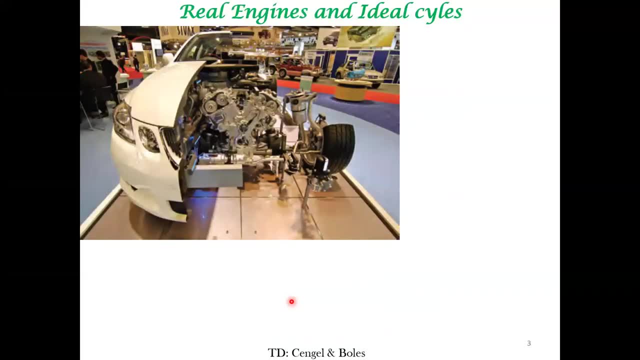 topic, which is analysis of power cycles. so you all seen power cycle, especially in the motorcycle or a car. so this is what is underneath a car: it's a, if you look at this, the engine, which is a very complicated machinery. okay, so gases are coming in, gas are getting out and lots of non equilibrium processes that do occur in real engines. however, 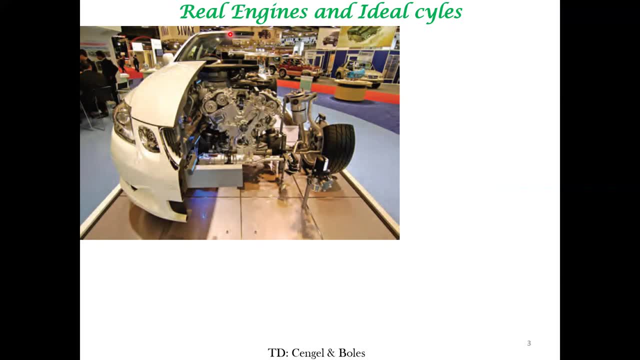 within the scope of this class, we want to analyze the working of power cycle engines using certain simple concepts that we have learned over this course. the real analysis of engines is made using fairly sophisticated computer simulations. okay, so it's a fairly complicated numerical problem using chemically reacting. 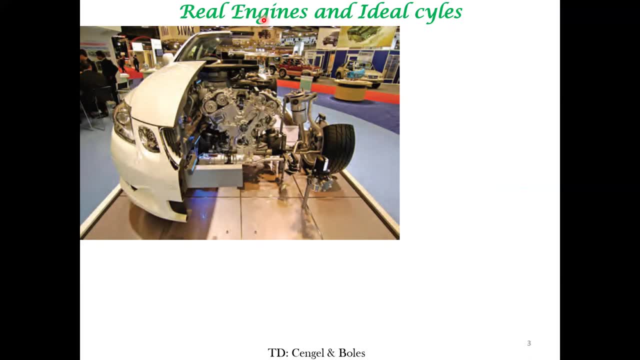 flows, computational flow, dynamics and so on. however, within this class, as we would identify certain features that are going to be used for analyzing these engines. so, if you look at all these power cycles, they are cycles, okay. so something occurs in a cyclical manner. so in the first half of the class, when we looked at like, say, Carnot cycle, we saw a fluid that undergoes. 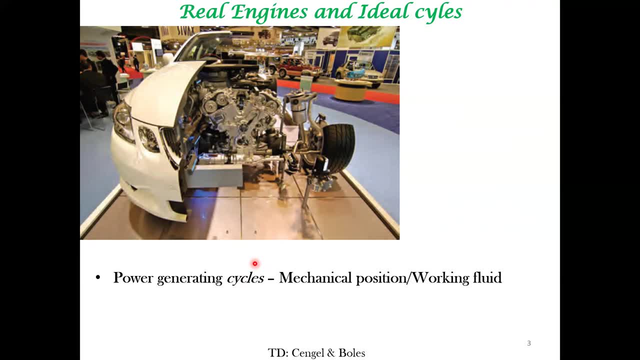 a thermodynamic cycle. often in these power cycle there is, uh, let's say, a piston. its mechanical position takes up a cyclical process- okay, so it can get go out off to get four freedoms, and sometimes it does come found down after several years, can reduce to many сыndrom 누� anytime. so it happens a lot. I was one of the. my days was a Yamaha technology machine. after the last, the first half, then i tired out, but it really cream. then, or attempt Kahnot side, we saw a fluid that undergoes the thermodynamic cycle. often in these power cycle there is, let's say, a piston. its mechanical position takes up a cyclical process, okay, so it can get low cycle and battering. você أ véritable, ä спортив, keine geh Онаρ. 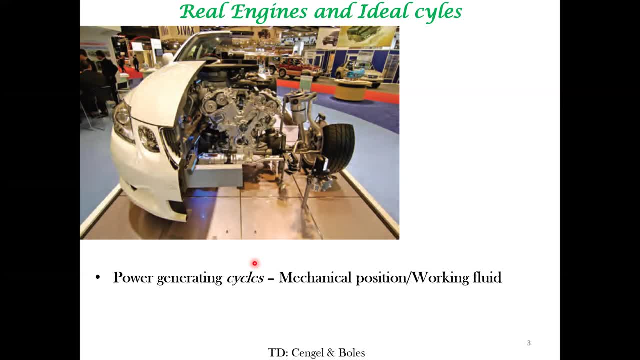 process. It can go up and go down. Mechanically it may take up a cyclical position. However, the working fluid, in contrast to what you saw in the Carnot engine, it may not have a cyclical cycle. That is, things can come and get combusted and get out The working fluid. 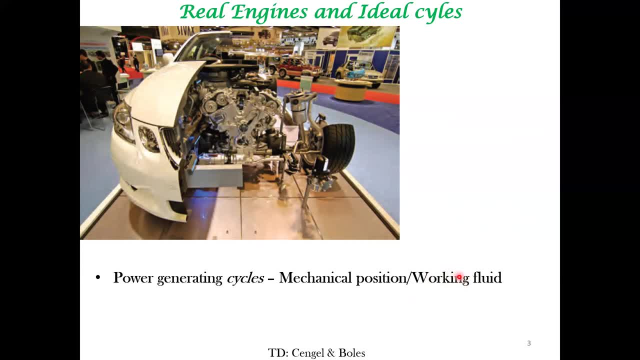 might not necessarily have a cyclical role, but the exhaust gases, once you exhaust them, gets the piston to the original position. There is a difference between the Carnot cycle and these kinds of cycles, Although both are cycles. you have to differentiate between these cycles. 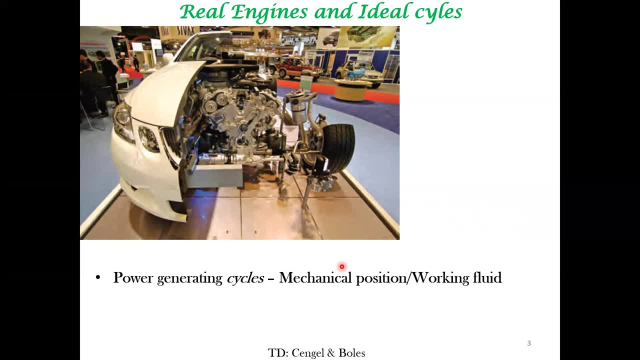 Here we are talking about some mechanical cycle. Effectively, some gases are taken in, combusted and thrown out, because of which the mechanical position is brought back to the original position. To analyze again this complex process, we undertake a viewpoint that things are operated. 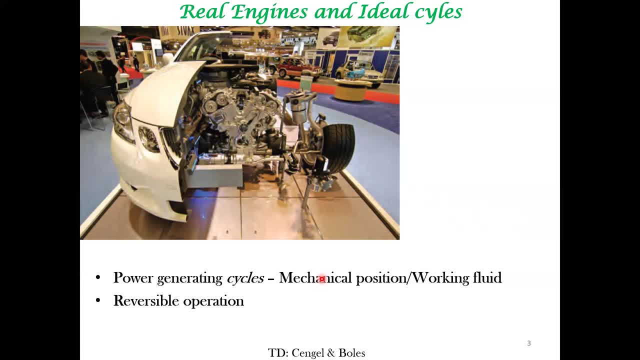 reversibly. Therefore, you can define the thermodynamic variables and then use quasi-static processes to analyze The real cycle. let's say, plotted in a PV diagram can be like this: However, we idealize them using certain approximations. It might be constant volume processes. 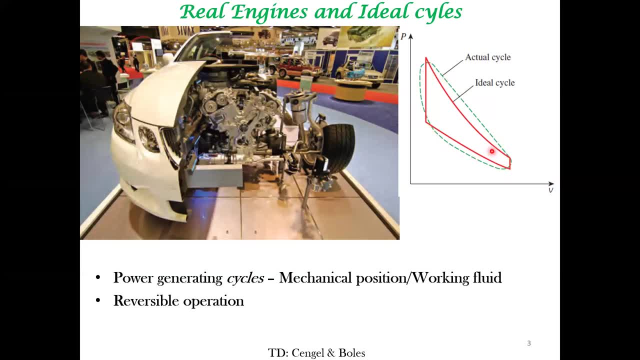 and so on. We use such analysis to look at the efficiency and so on. We will clarify as we go along what kinds of approximations we use. Eventually, what is the question we are trying to ask? We are trying to ask the question of efficiencies. What is the network that is? 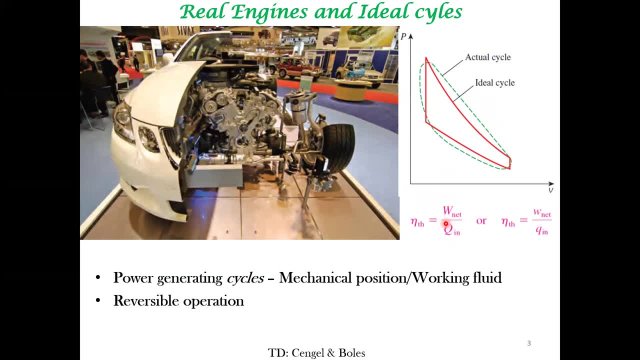 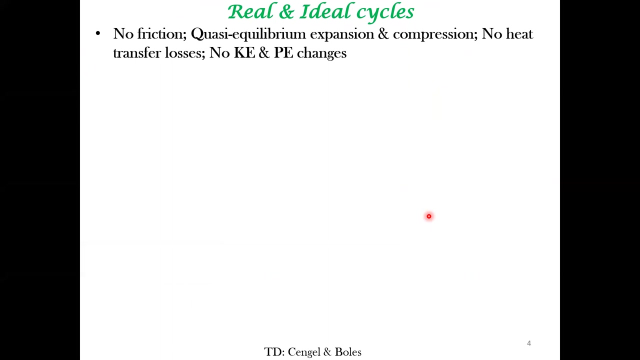 generated, divided by what is the heat input. The heat input can be of different kinds. We will look at these different options available to us. Finally, we are looking at some kind of measures of efficiency for the operations of these engines. This ideal and real cycles differ dramatically. To make analysis possible, we use a range of 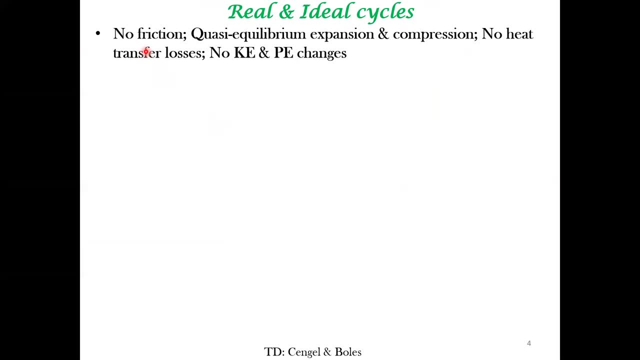 approximations. First, there is no friction, You have quasi-equilibrium expansion and compression. There are no heat transfer losses, You neglect kinetic and potential energy changes of the fluid, and so on. These look like drastic approximations. Maybe they are too Within the scope of this class. 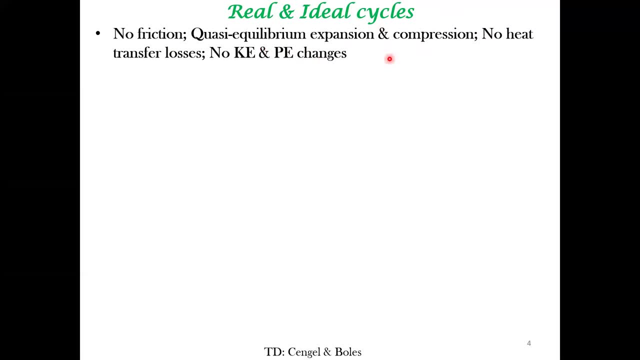 to make analysis possible. these kinds of approximations have to be utilized To look at the work and heat interactions we plot in these processes, such as the cyclical process. This will go from 1 to 3 to 4 and 4 to 1.. 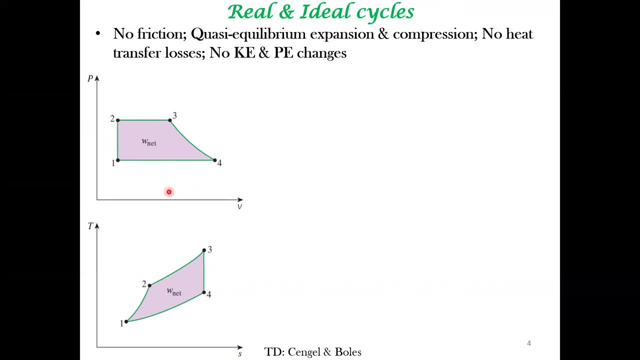 The plot in the p-v diagram. that helps us get the network interaction. The T-s diagram will give you the heat interactions also. All these things you can connect to the make sense of all we are talking about, all the processes which we are talking about here. you can. 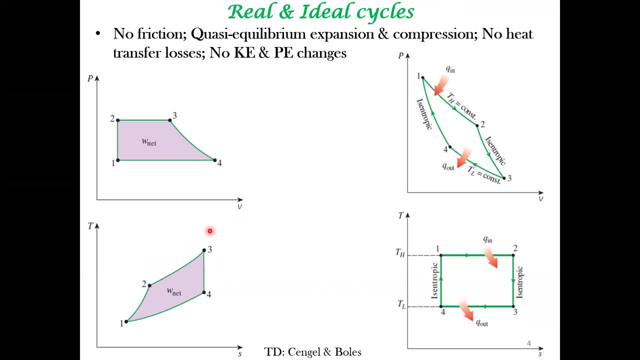 connect these things to what we have already looked at in the Cardinal analysis. Cardinal analysis was a cyclical process. There was a fluid that had a thermodynamic cycle. It had two heat transfer process and two work transfer process. We could plot all these information in. 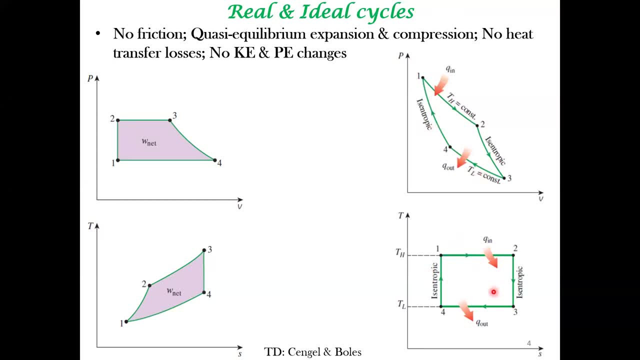 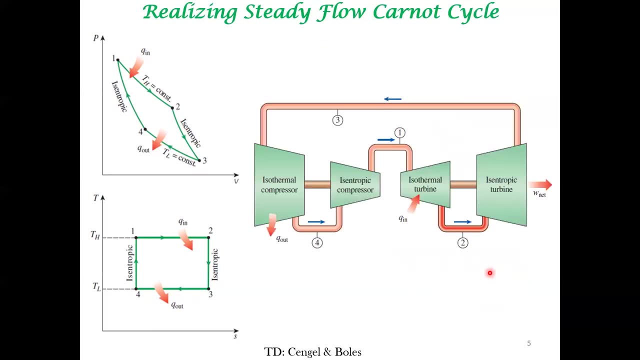 the P-Way diagram and the T-S diagram, which helped you assess the work interaction as well as the heat interaction. And you can- though it looks abstract, you can- realize a Carnot cycle. In this cycle it's a fluid is being 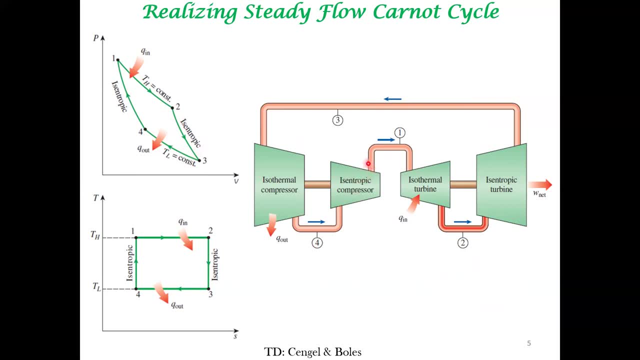 circulated right. So the fluid, there's no intake or exhaustion, There's no intake or outlet of fluid. The same fluid is being circulated across the different processes. For example, you may start at, let's say, process point one, state point one which 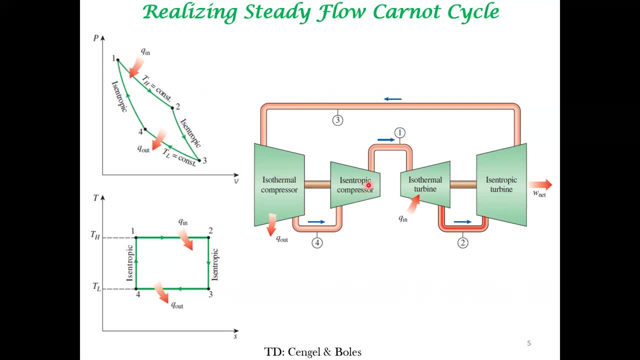 corresponds to this point. And there is an isothermal turbine which gives rise to expansion, And you end up at this point. Then there's an isoentropic, there is a turbine which generates work, And then you come to state point. 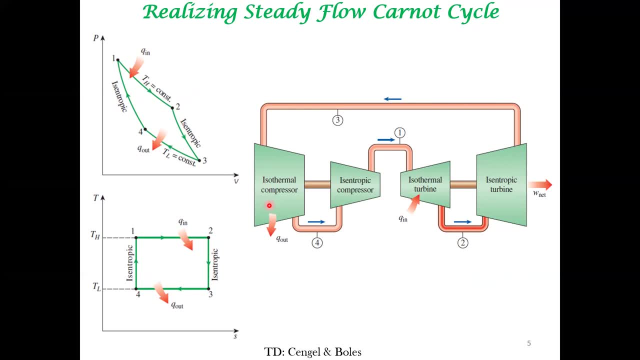 three, which is here, And then there is another isothermal compression which releases heat, and there is an isoentropic compressor, And so on. So in this steady flow, slow Carnot cycle, the expansion and compression is driven by turbines and compressors. 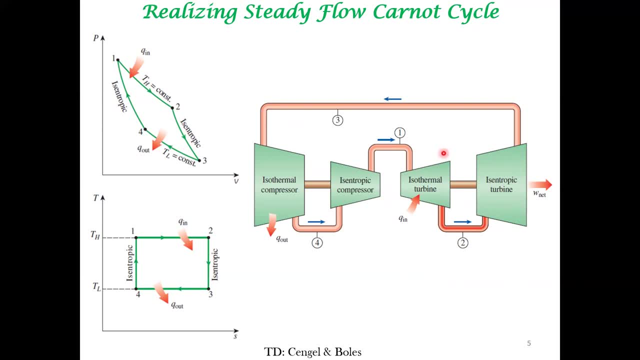 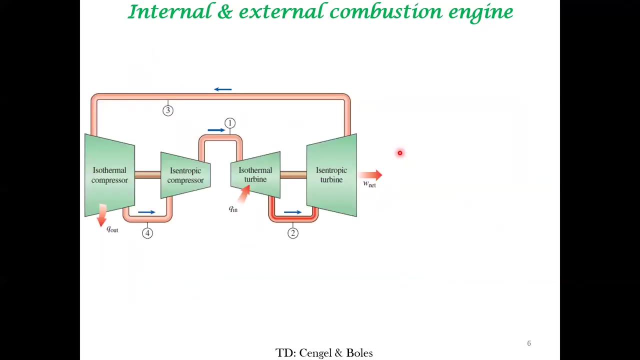 And the same fluid is being circulated all around, Right? So even though this looks abstract, it can be realized in a turbine and a compressor. So there are. we want to make sure that there are no barriers to combustion reaction, in case you have any problems with the engine. 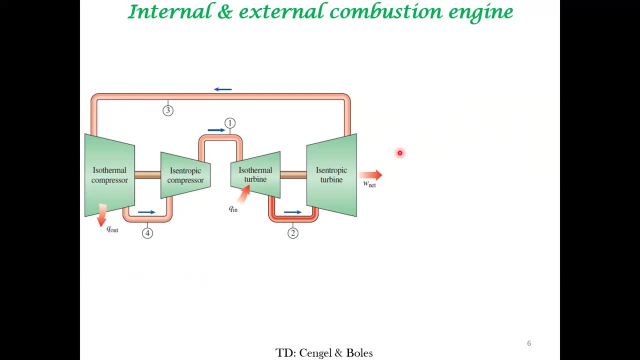 And so at the stage of this, there is no sectional combustion engine. the combustion engine is not something that should be in your oil-fired engine. The combustion engine has to be in a combustion engine. So if you want to differentiate a particular terminology, 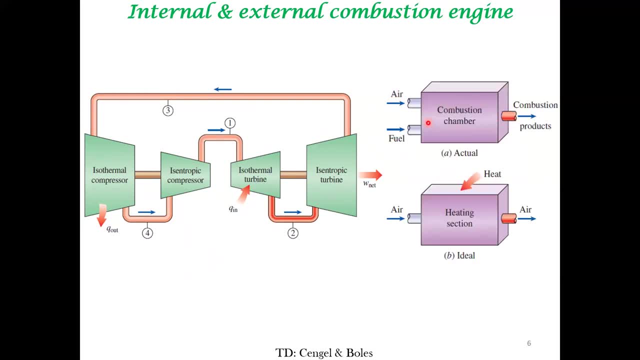 you might have heard about internal combustion engine. right in your motorbikes and cars There's an internal combustion engine, But in this case, is what we are looking at given to the heating section in an internal combustion engine? uh, let's say what you see. 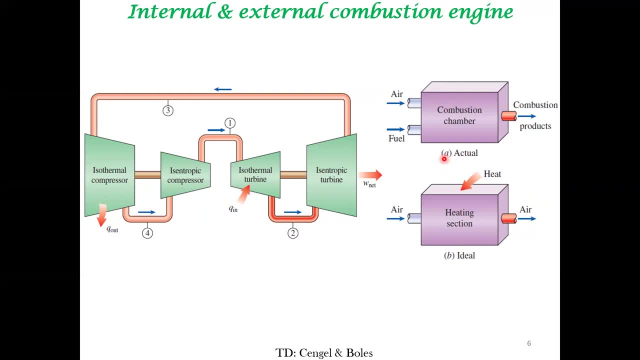 in your motorbike, for example, there is fuel, there is inlet for a fuel and there is air. also, there is taken in. both of them combust, uh, this combustion that occurs and heat that is generated- all that might occur internally within the engine. okay so, but as opposed to an internal combustion engine? 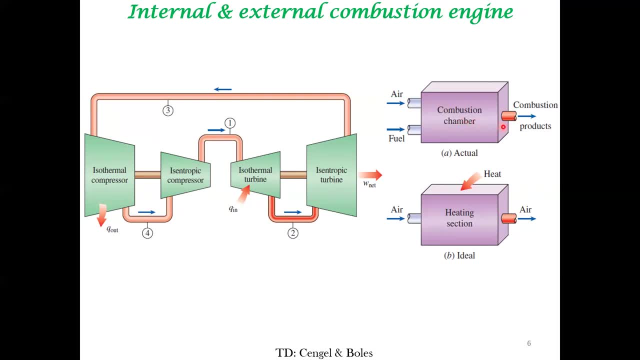 where combustion occurs internally. heat is generated internally and there is an exhaustion of combustion products. to get you back to the mechanical cycle in external combustion engine, the combustion occurs externally and that heat that is generated is given to the heating section. so this might be the actual, real process. okay, but this process is very hard to understand. 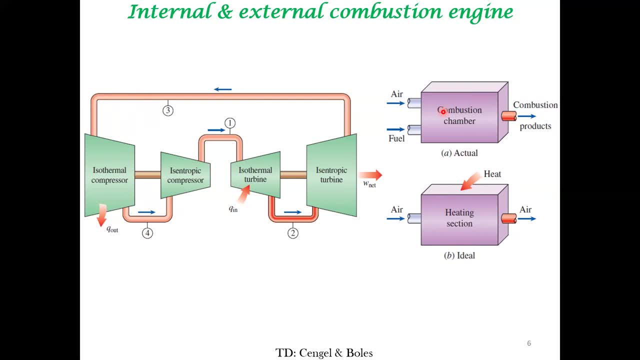 it's not a closed system. so what we end up analyzing is the closed system. okay, so this is a flow system, things coming in and things getting out- but we do not really analyze this internal combustion engine. uh, so we take an equivalent, or in what way they are equivalent, supposing you have heat, that is. 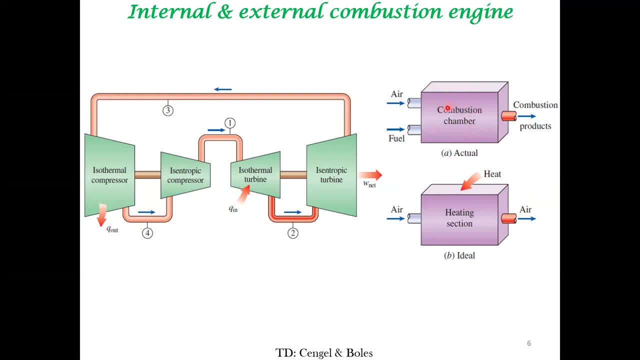 being generated. the amount of heat that is generated by combustion is the same as the amount of heat that is being given in. in that way they are equivalent. and then you ask: given this heat input, how much of work can be generated? is you ask some such question? 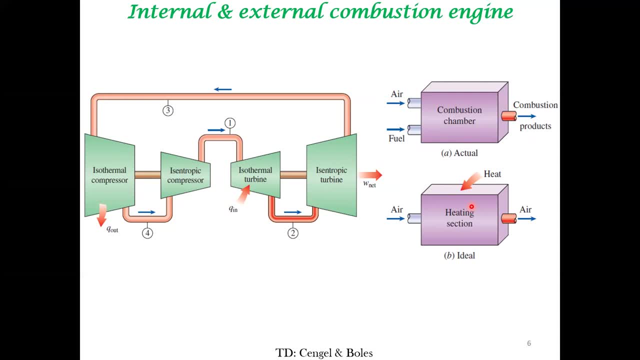 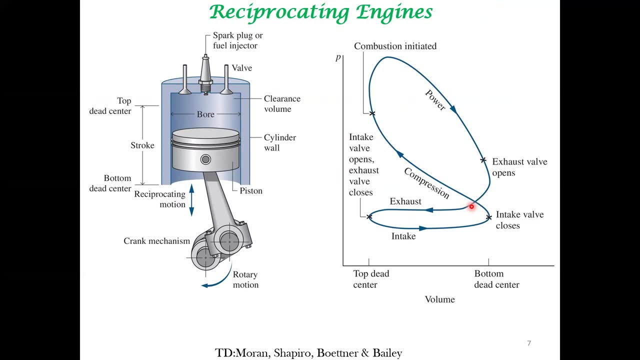 when you analyze the combustion engines to make all these things possible, the machinery that is used are what are called reciprocating engines. so this is an engineering marvel. i would say so we will, all the reciprocating engines. what it manages to do is it is able to convert a cyclical linear motion into rotatory motion. right, so this is connected. 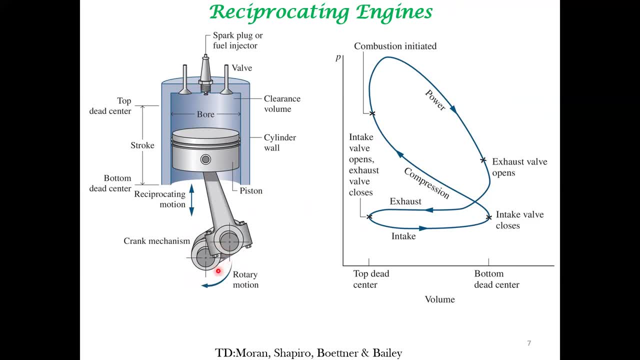 to a wheel. so that is a very interesting way of being able to translate what appears to be a linear, linear motion into a rotatory motion. uh, rotary motion, okay, so let us. it is. these much reciprocating engines have different components. there are valves. this can be the inlet valve for letting in uh air and so on, iron fuel, and then there can be 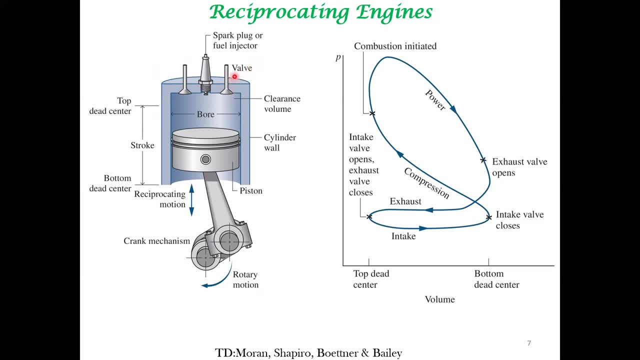 an outlet valve for letting out the combustion products and there can be a spark plug. this is spark injected, uh, spark ignited. reciprocating engine. then there are two major kinds. one is spark ignited, another is come, uh, compression ignited. we will see the difference, why one is more efficient than the other. 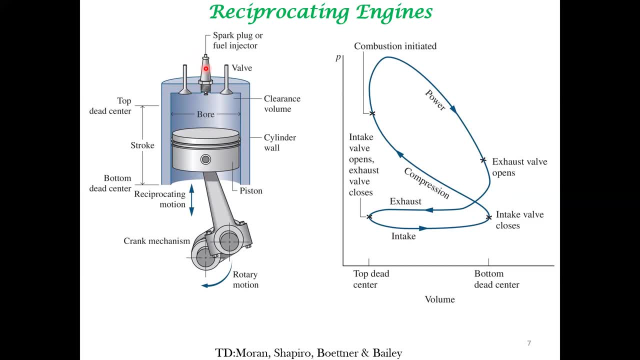 and what is the advantage of, let's say, spark ignited as well as the comp, uh, compression ignited engines? so this, and there are some terminologies- there is this top dead center when this piston is at this position and the piston when at this position. this is called the bottom. 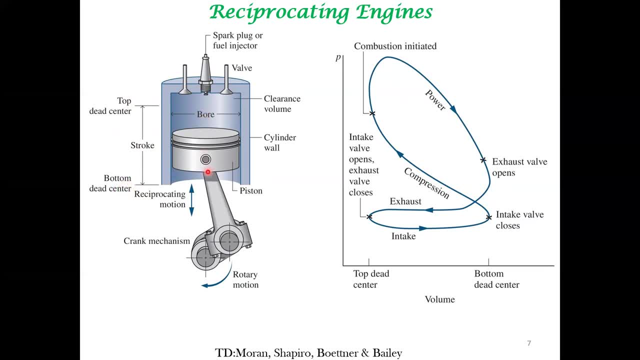 dead center. this distance it travels, this piston travel is called stroke. okay, so you might heard something called a two-stroke engine, four-stroke engine, right? so in a two-stroke engine, for for one cycle, it uh one rotary motion, there are two strokes in the engine, uh this. 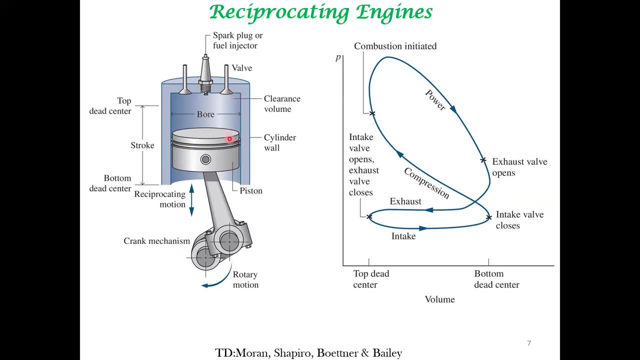 and there's a piston, and there is- uh, it is all. this piston is enclosed in a cylindrical one, right? so typically the way this reciprocating engine works is: you start. there are four segments to the entire cycle. you start at one point. okay, so this point is typically, let's say, you take at this point intake stage. okay, so the pressure is. 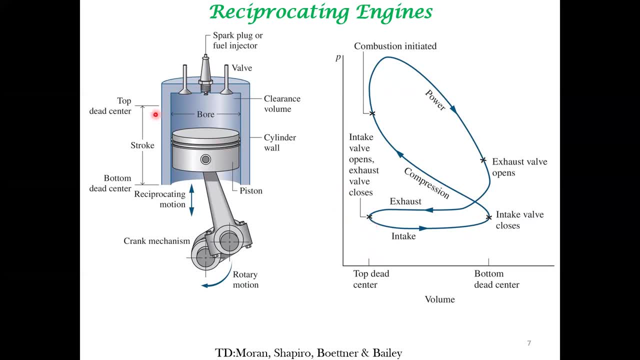 less and this piston is at the top dead center. okay, so that is the volume. so the inlet valve opens and the exhaust valve closes, right, so this is closer, closed, and let us say this is the inlet valve that is open, So it lets air and fuel in. so 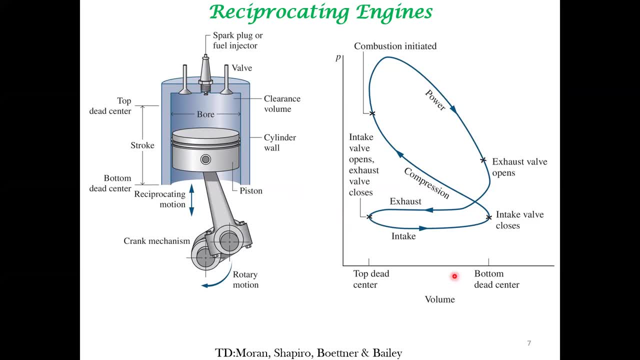 the piston moves down, the volume increases, it goes the inlet stage. it goes all the way up to this point. okay, where the piston has reached at this point, this closes, all right. So, and then the inlet valve closes, then it starts moving back, the volume decreases. so 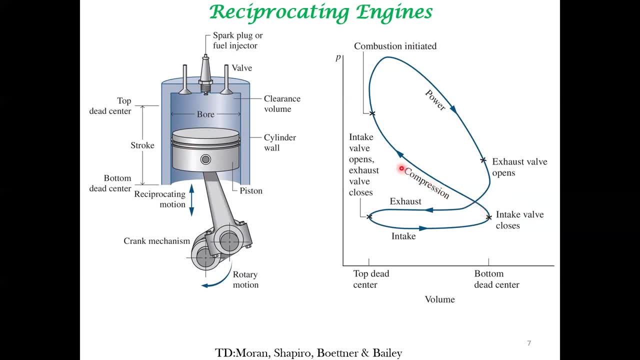 this is called the compression segment. So, as the air and fuel are combustion, there is an ignition because of the spark that is generated by the spark plug, And then There is a sudden increase in pressure, Then this is the most important segment where work is being generated. it's called the power stroke. 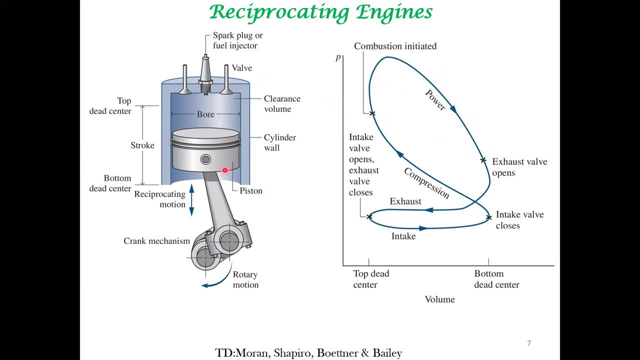 okay, So this moves down, the piston moves down, the volume increases and then, beyond a particular point, the exhaust exhaust valve opens. at this point this is the exhaust valve that opens up and is channeling forward a little bit, And then all the combustion products are taking. 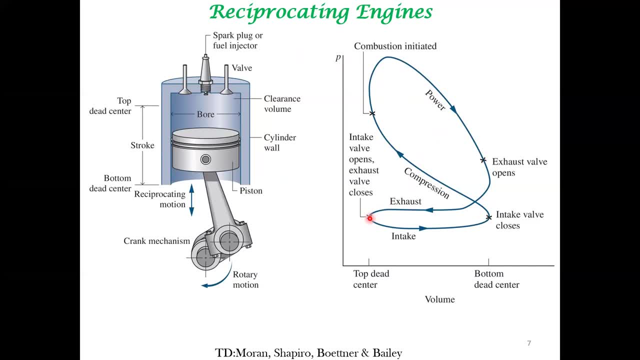 out of the system. it's so exhaust thing gets out to the system And then you come back to this point. okay, so ICP, that's one way to remember intake compression power at exhaust. okay, ICP, these are the four segments. offer engine produced again. 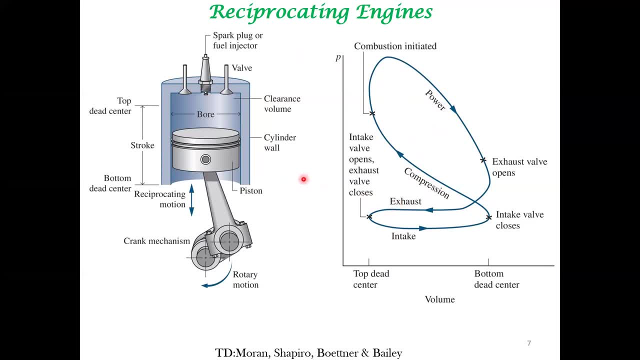 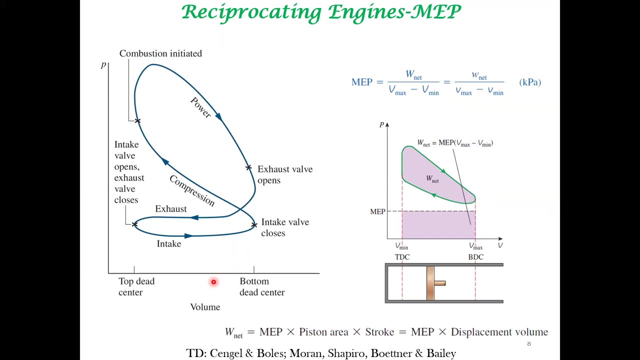 r, okay, which enables this cyclical linear motion to be translated into a rotary motion. okay, so it's a. it's a really amazing um device. all right, so we will analyze this device. okay, there are variations to this device and we will look at this in the next few classes. takes you lectures, so there are more terminologies. 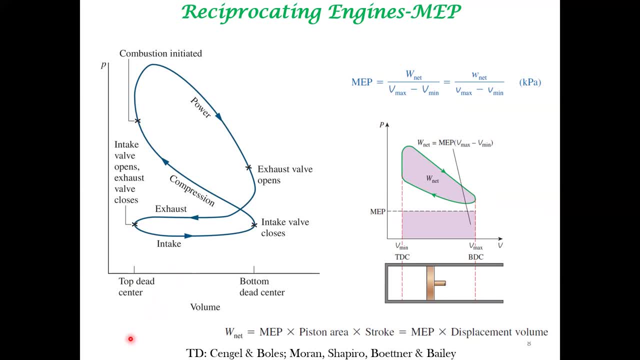 you ought to understand. there is something called mean equivalent pressure. okay, so what is that? okay, so the work you obtain from the reciprocating engine is this work. what is mean equivalent, uh, pressure? so you take this work and divide it by this change in volume. okay, so this is. 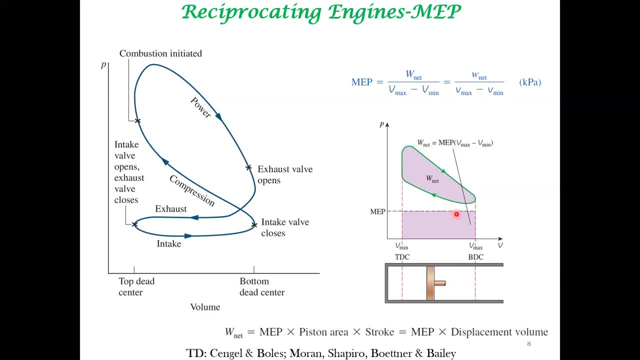 the constant pressure that is present in the power stroke. okay, so higher the mean equivalent pressure, the work that you can obtain is greater. okay, so this is the definition of mean equivalent pressure, because that tells you for a particular engine. the engine is defined by the different these two volumes: right, maximum: 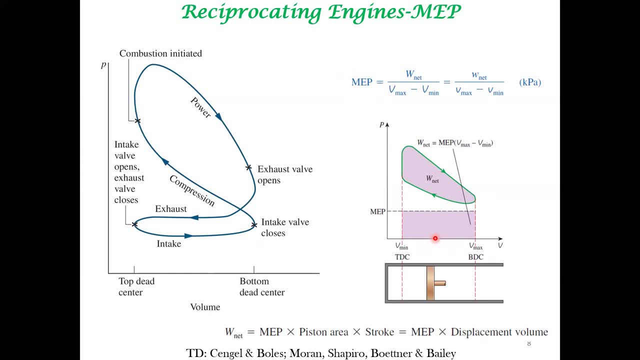 volume and volume difference between top and bottom dead centers. once this is fixed, the higher the mean equivalent pressure, the greater is the work that you can obtain here. engine, so the total work that you can get is mean equivalent pressure. piston area times stroke is this distance travel. so this gives you the volume, so mean equivalent pressure. 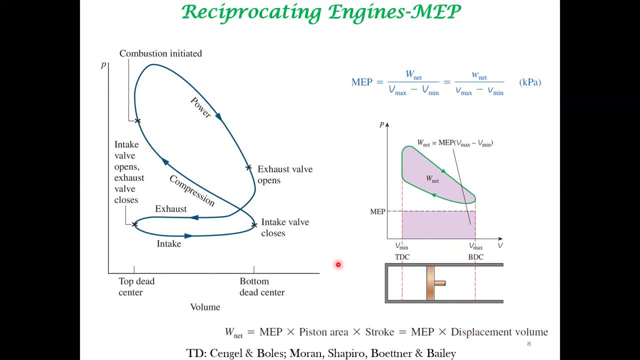 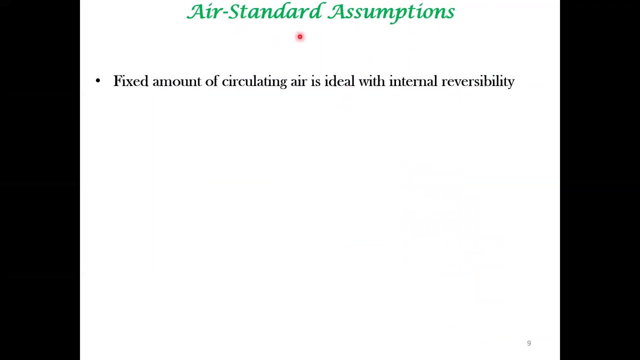 types, the displacement volume. as i said, the real process is 선 am the efficiency of cycles. So all these things are clubbed into what is called the air standard assumption. Instead of looking at inlet and outlet of gases, you look at a fixed amount of circulating. 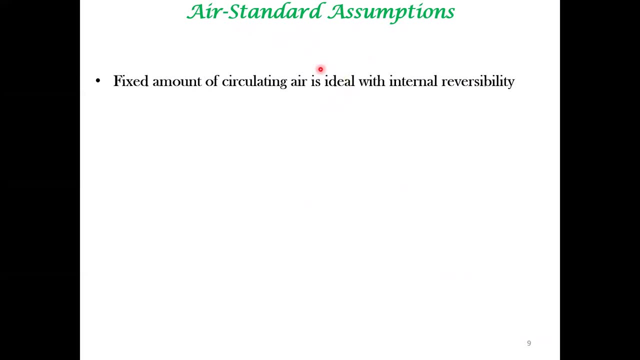 air- That air is also considered to be ideal- and all the processes that occur within this fixed amount of air, which makes making it a closed system. these processes are internally reversible. We also consider the heat that is generated via combustion is added to a working fluid, So that's. 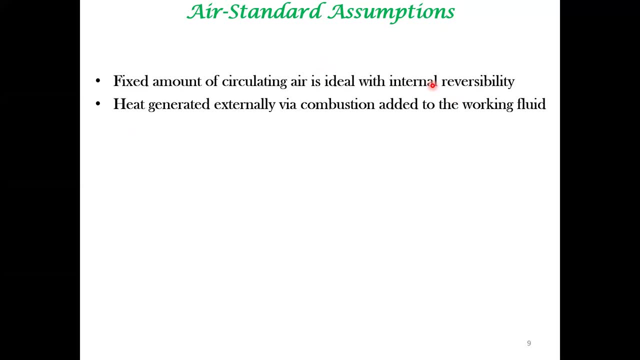 the way we add the heat that might have been generated externally, for example in an external combustion engine, Or the heat that is generated internally in an internal combustion engine. this heat is added to the fixed amount of circulating air In a real process. the exhaust of the combustion products helps you get mechanical. 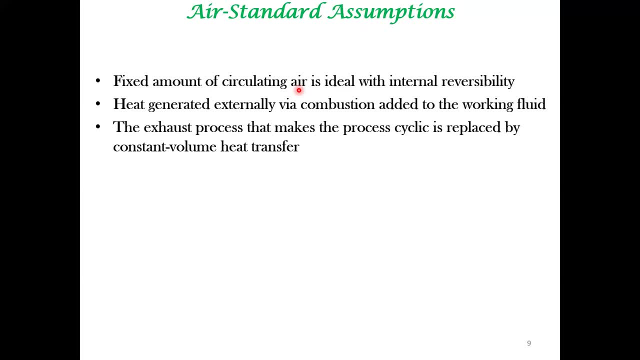 cyclability. it gets the piston to the original position. Okay, So we don't really consider a flow system. there is no exhaust, there is no process corresponding to outlet of combusted products. Instead of that, you replace that process by a constant volume heat transfer, which. 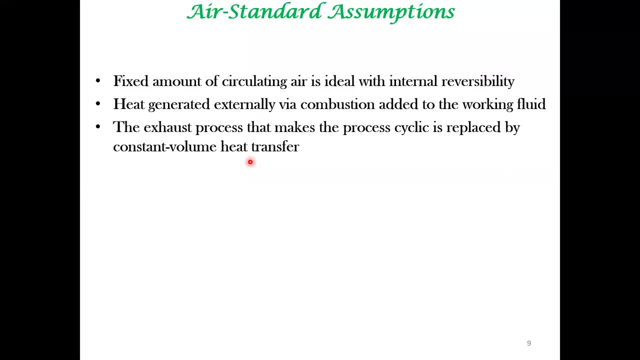 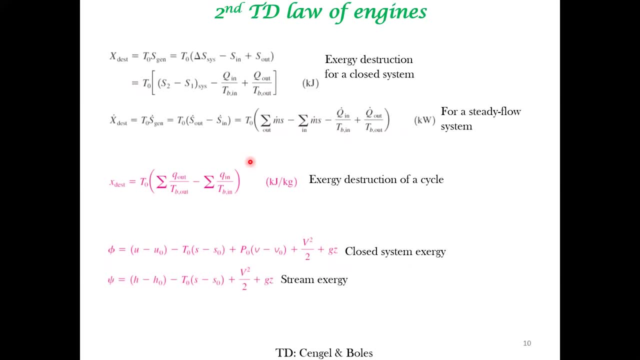 makes mechanical cyclability okay. it gets the piston back to the original position. With all these things, you apply the first and second law and the exergy analysis which we have already seen right. So instead of looking at a flow system, okay, a certain power cycle flow system is also. 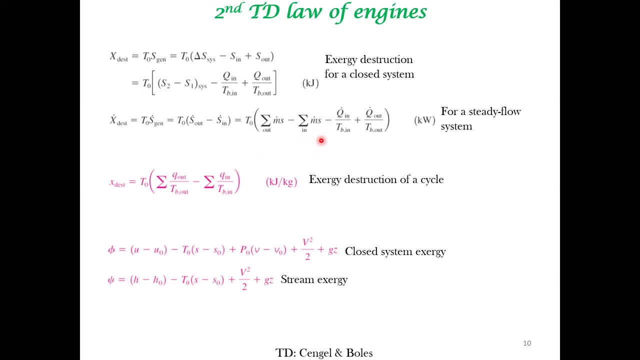 will be looked at, but typically all the laws that we'll be using- the first law, second law, the exergy analysis- will be for a closed system. We have already done this analysis Or stated the equations that are relevant for the analysis of a closed system. in many 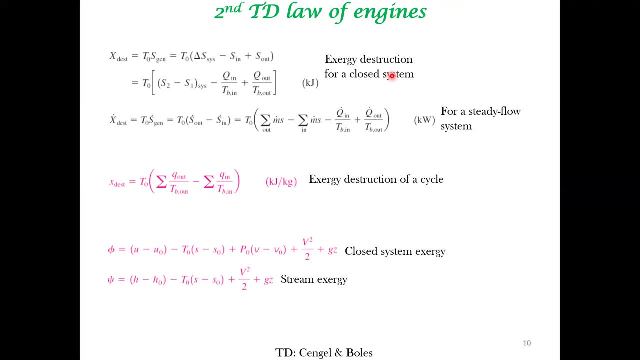 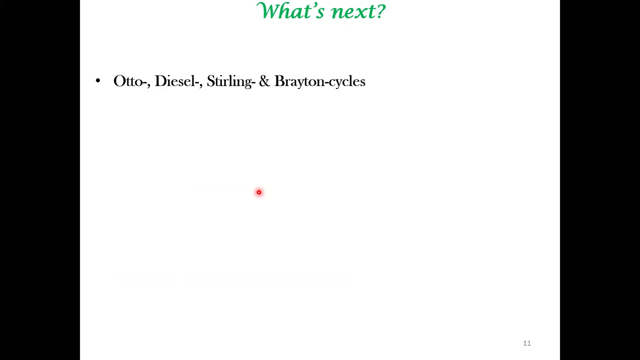 of the previous lectures. So those are the equations that are going to be utilized for looking at the different power cycle. So in this first lecture there's an introduction to what is called gas cycle, That is, The circulating fluid doesn't change any, change its phase. okay,